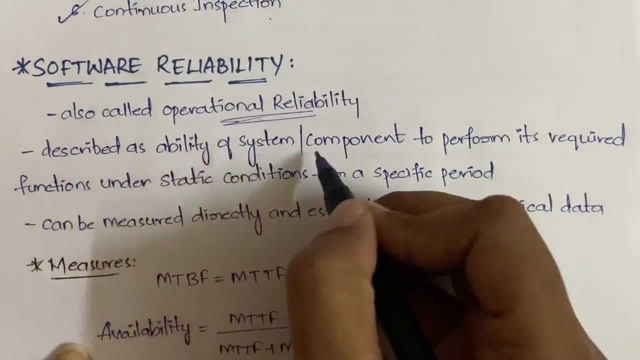 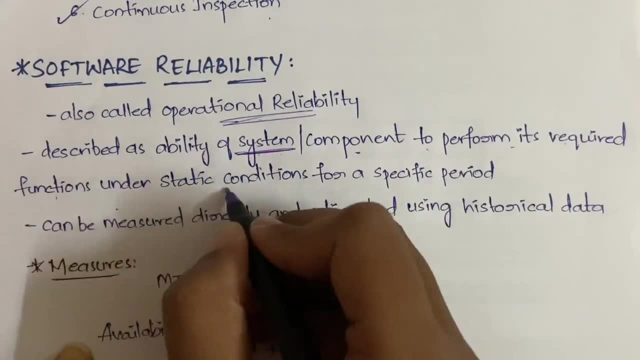 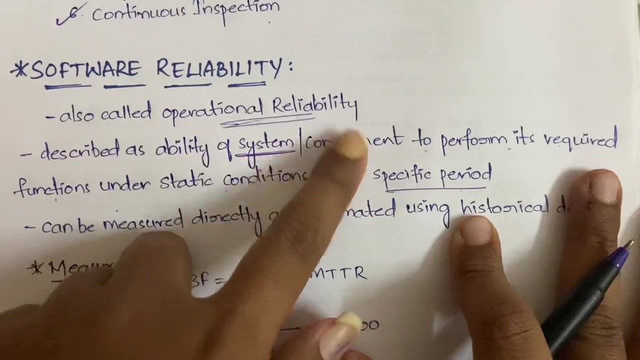 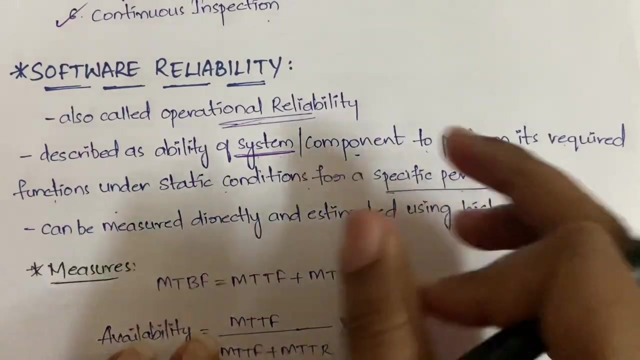 Very simple. It is described as the ability of the system or component- ability of system, let us take- to perform its required functions under static conditions for specific period. See, don't get confused. It is described as ability of a system or a component- anything, ability of a system to perform its required functions. that is what functions it is supposed to perform. Those functions will be performed under static conditions, that is, there is no change in the conditions. 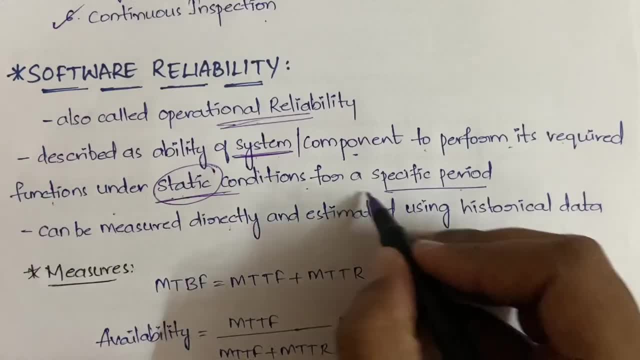 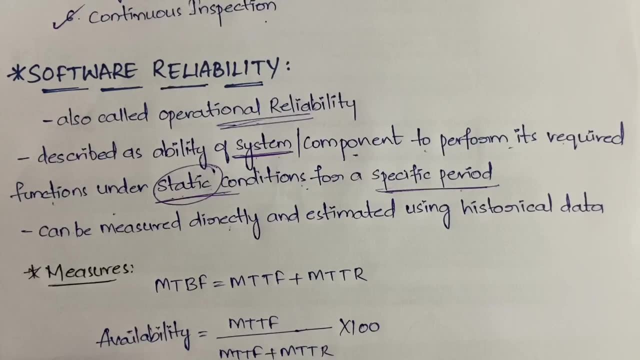 The conditions will remain same, Got it. And conditions for a specific period. that is, only for a specific period, not it? not throughout its lifetime, Got it? So it is described as the ability of a system to perform its required functions. that is what it what it is supposed to do, all those things it has to do under fixed conditions, static conditions for a particular period. Very simple, Okay, And it can be measured directly and estimated using: 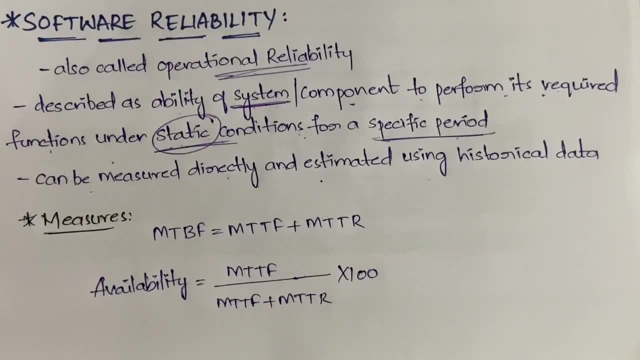 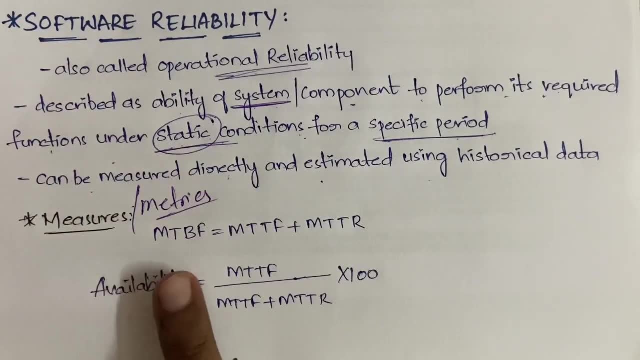 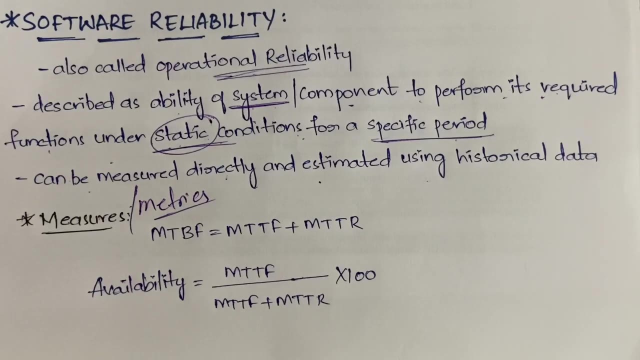 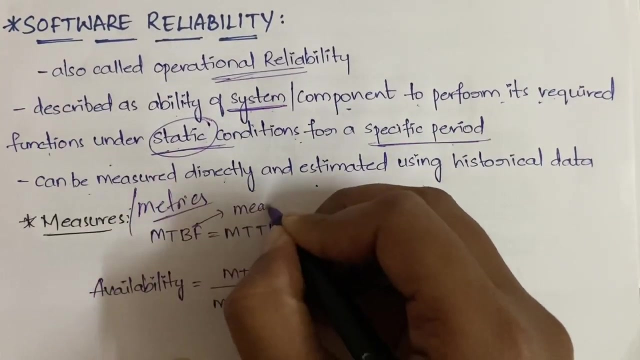 historical data. Okay, Now what are the measures? measures, or you can also say metrics also. So what are the metrics of this software? reliability, then see, MTBF is equal to MTTF plus MTTR. No, don't get confused, I'll tell you what is MTBF, MTTF, MTTR? So MTBF is nothing but this one mean time, mean time between failure. 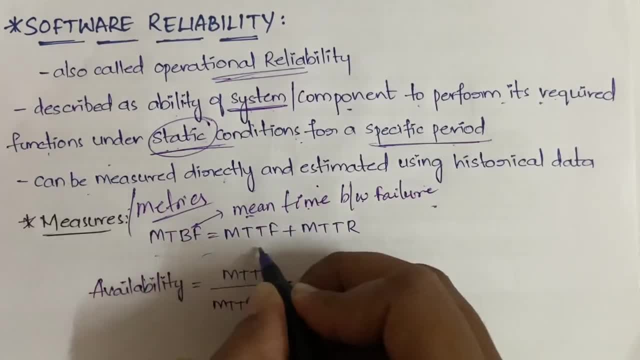 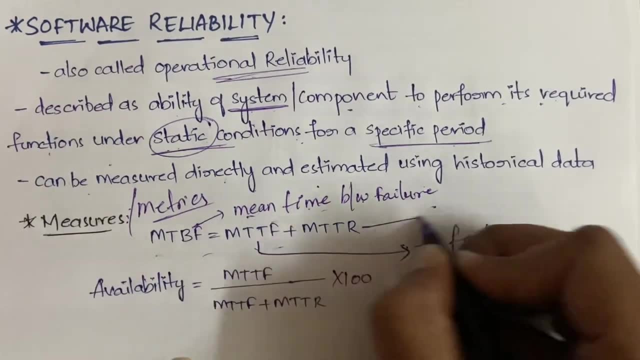 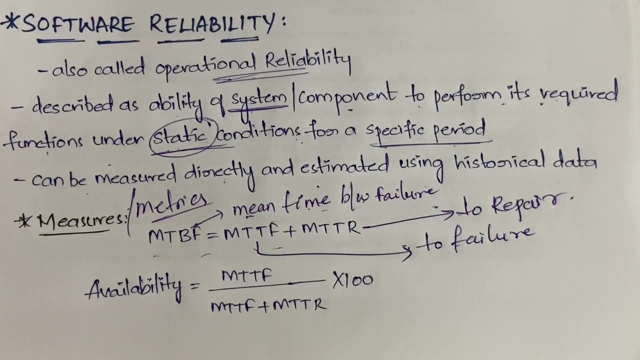 Okay, Maintime between failure, MTBF and MTTF is nothing but mean time to failure, Mean time to failure and M GTahren is nothing but mean time to repeat. Okay, So this is these are the metrics and other metrics also We have. availability is equal to MTTF by MTTF vs MTTR into 100. Got it. So this is about software. 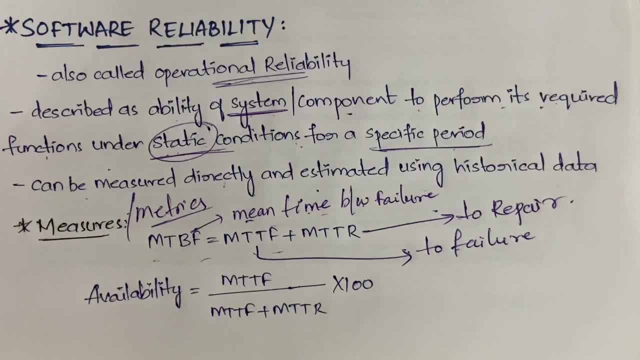 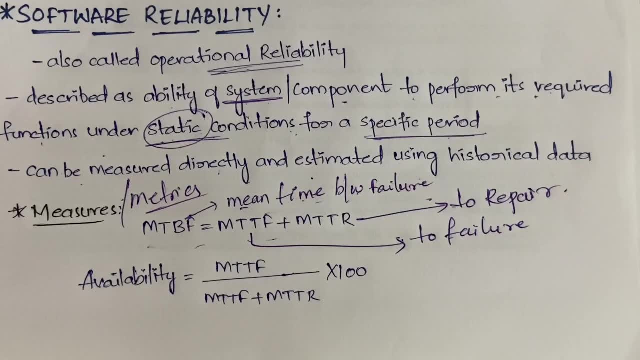 reliability. very small concepts, Very easy concept, It is very simple. It is described as the ability of the system- or probability of the system, also you can say- to perform its required activities. it required functions under fixed conditions over a particular period of time. and these are the sorry and these. 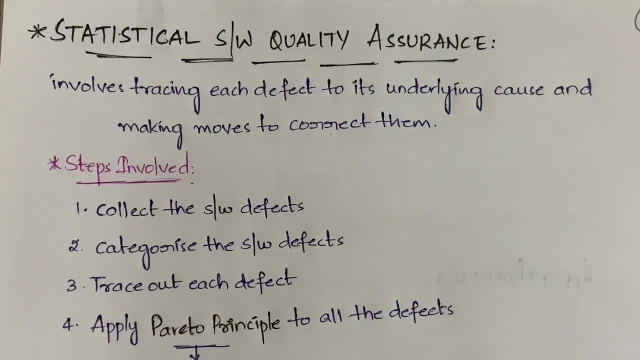 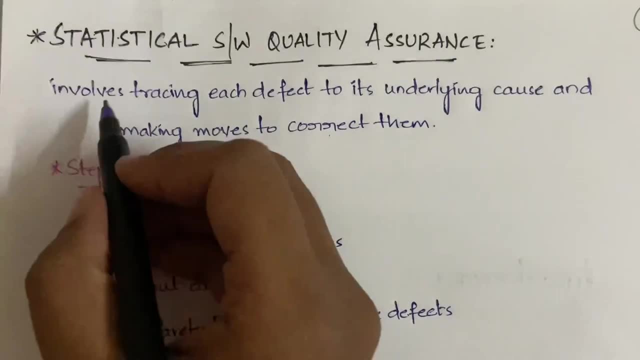 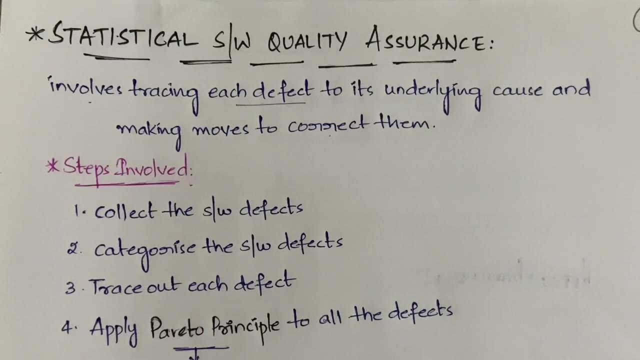 are the metrics associated with the software reliability. okay, now let us discuss about the statistical software quality assurance. again, this is very easy. so first of all, it involves the tracing of each defect that is, in your software, or in your product or in your application website, whatever it is. but since the subject is software engineering, so in your software you will. 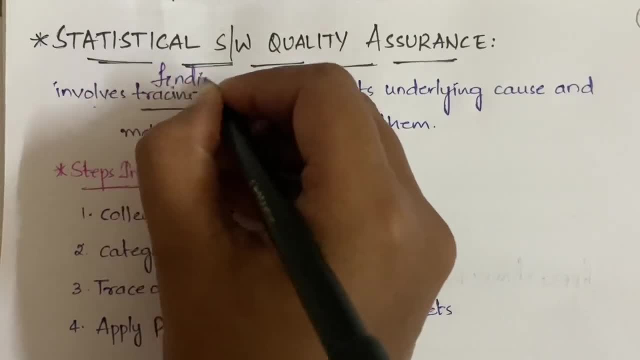 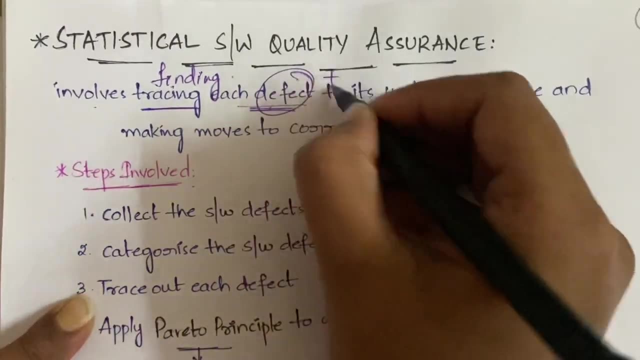 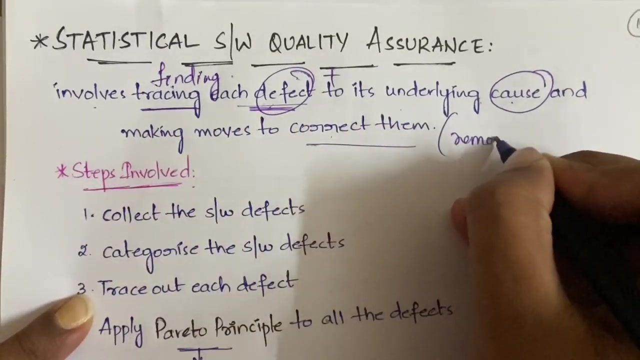 be tracing out, that is, find out, finding out each and every defect to its underlying cause, that is, the defect plus the cause why the defect has occurred- and making moves to correct them, that is, to remove the defect got it. this is what statistical software quality assurance deals with. 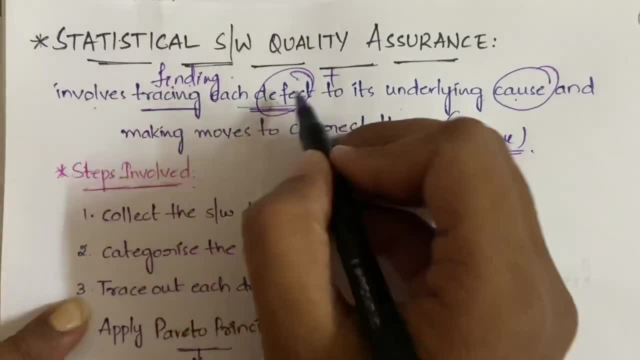 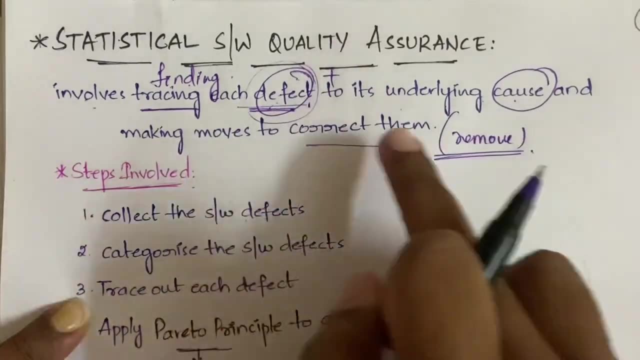 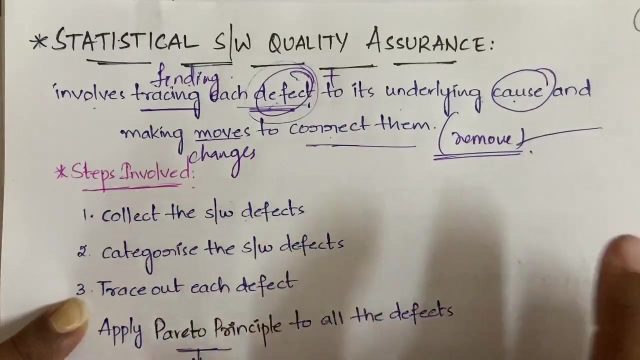 okay. so it involves you finding out each defect- that is, what are the defects, as in our software, along with their causes- and making some moves, making some changes- you can say making changes- to correct those defects, that is, to remove the defects. got it now in this statistical software: quality assurance. 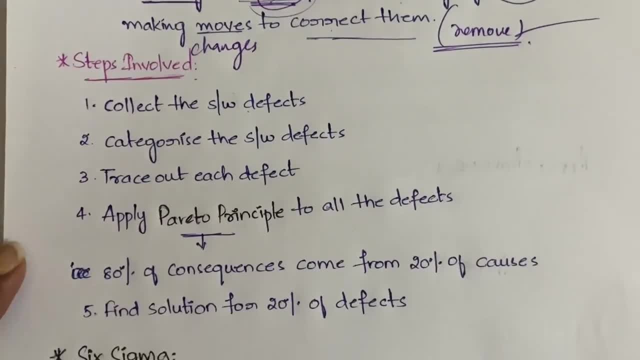 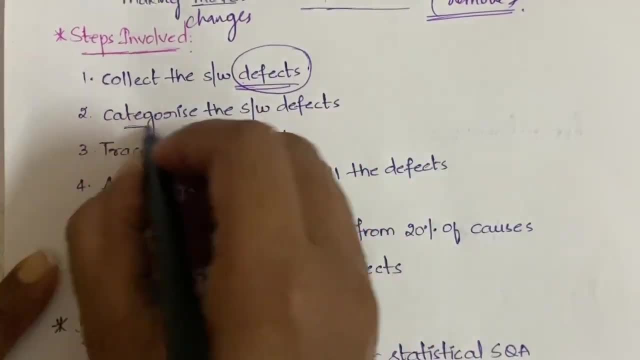 what are the steps involved? I'll tell you now. first, what you have to do is you need to collect all the software defects. okay, so first collect all the defects which are present in your software and reconfigure them to the software. you need to categorize all the defect. ok, make sure that. 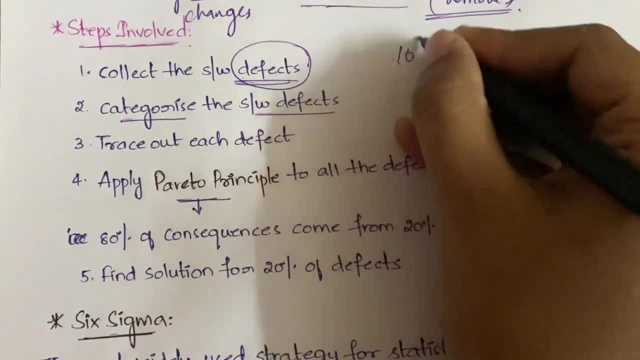 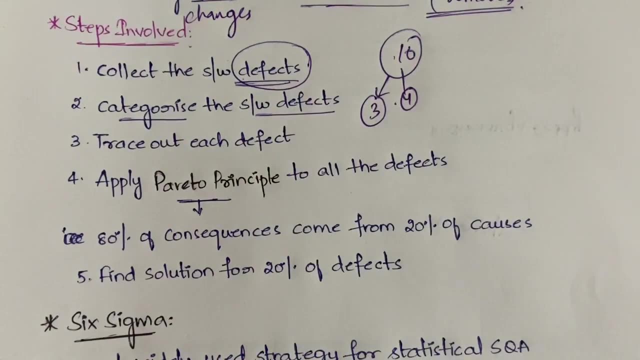 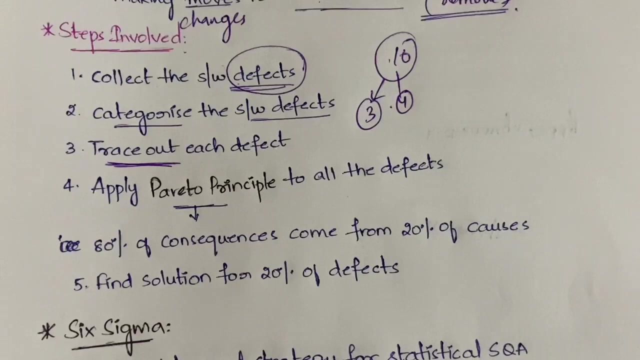 you have them sorted and categorized and what you need to do is find out where each defect is, such as alternative defects, reflector defects. one thing which is important about Yoon's system is that you need to categorize each defect First of all. once you know you need to categorize these defects, which are proper defects, then 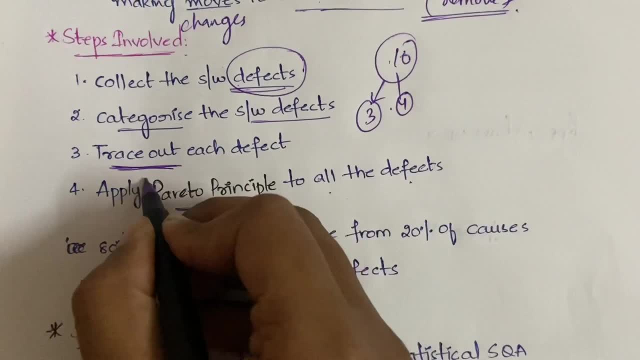 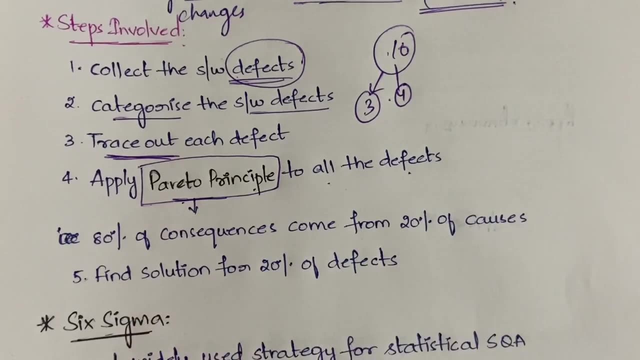 the next step is start the process. so this is what you need, first of all, to drive a software. Pareto principle is: 80% of the consequences come from 20% of the causes, that is initially, for example. I'll tell you. let us take an example of a tree or anything. it could be okay, let 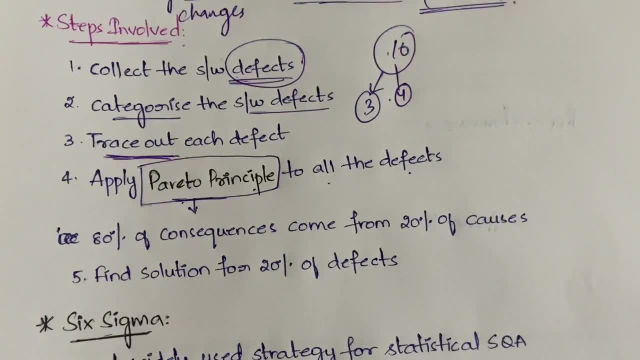 us take an example of coronavirus itself. so initially in our body, when we are infected, initially we will have only few virus right in our body, like we may have some thousand to thousand, thousand, two thousand virus particles in our body, if it is, if we could not find 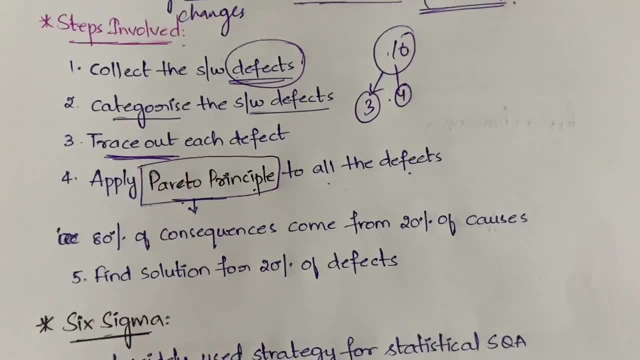 it out if we left it in the same way. by two or three days it becomes 10000 or 20000. by five, six days it becomes some lakhs. so it develops right. because of one single virus particle, so many virus are developing, so many particles are developing. so here also in the 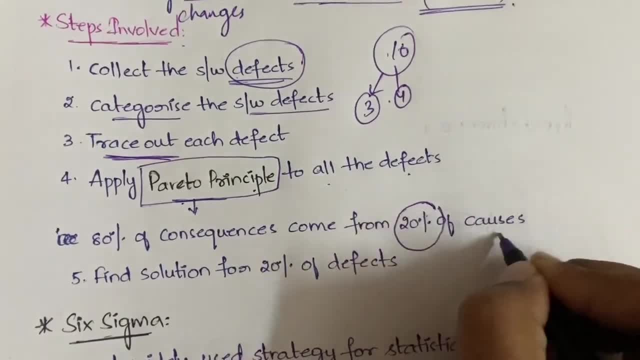 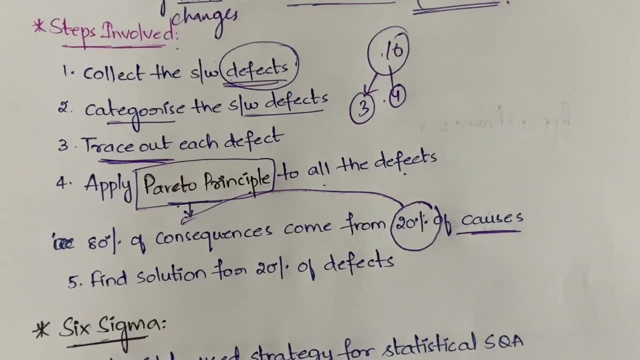 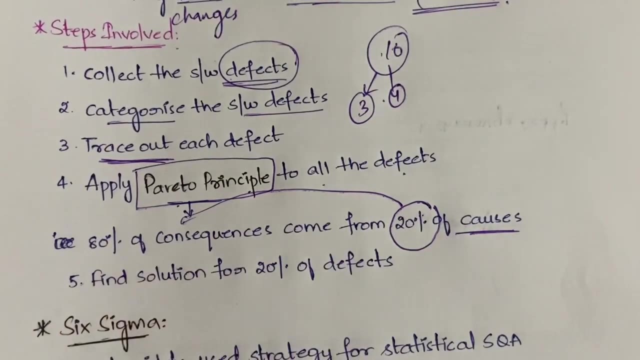 same way, because of 20% of causes, these 80% are coming as consequences. because of 20%- 20% of defects, the remaining 80% defects are coming as consequences. You know what is the difference between cause and consequence? right, Cause means the reason why it has occurred. 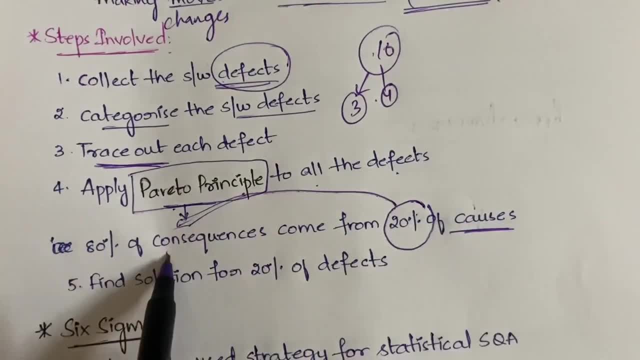 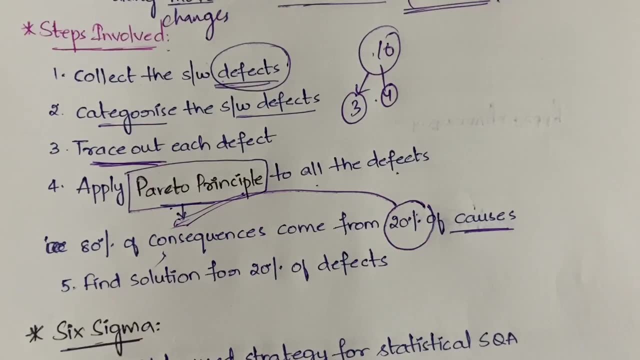 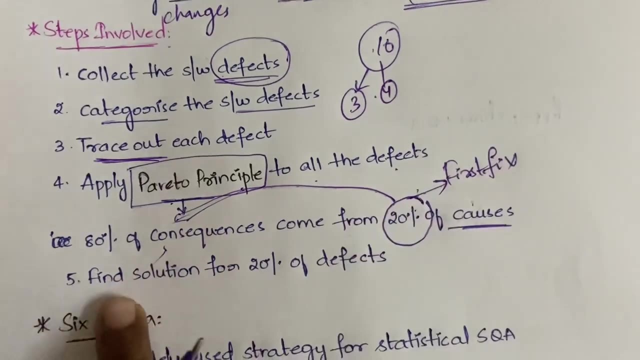 Consequence is the consequence of this. the result of this Got it. So, because of 20% of the defects, the remaining 80% are coming. That is what Pareto principle means. So, first what we have to do, we have to fix this 20%. First, we need to fix this, Find out solution. 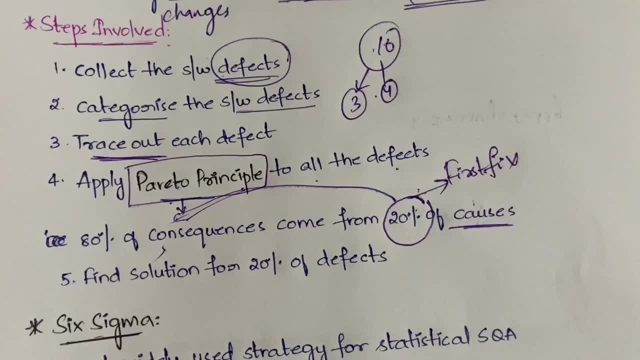 for 20% of this. First, we have to fix that. If that is being fixed automatically, 80% of the defects will not come right. If that is correct automatically, 80% of the defects are. 80% of the consequences are fixed, Got it? So this is what Pareto principle means. 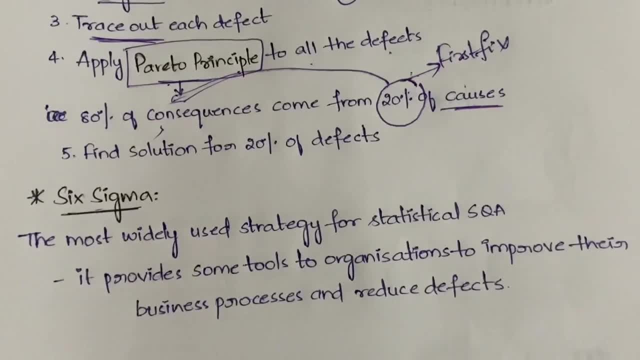 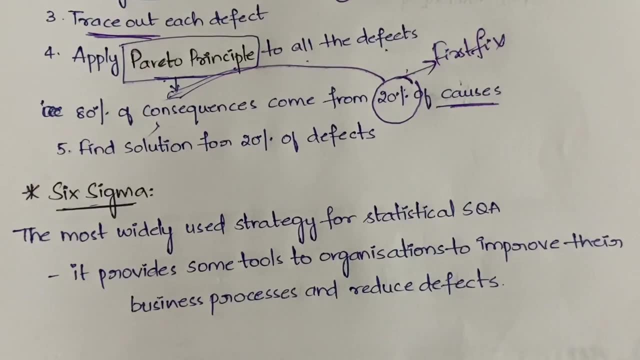 Right In this we also have another concept, that is, the concept of Six Sigma. So basically Six Sigma. you might have already known about this. I already made a video about Six Sigma in management sciences playlist. I will give the link of that in the description. You can check it out there. I am not explaining it. 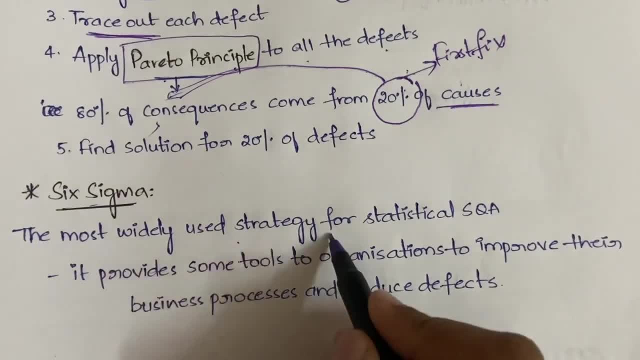 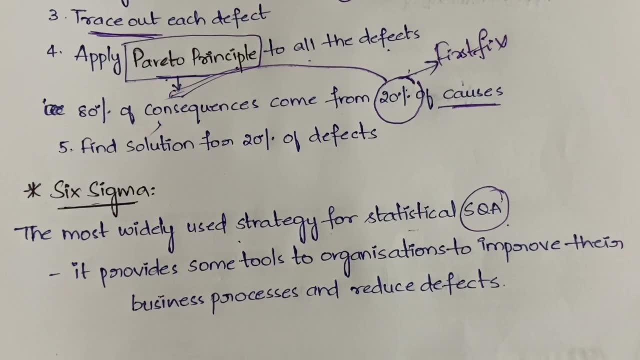 again because I have already made a video. So Six Sigma is the most widely used strategy for statistical. SQI means software quality assurance. Okay, So it is the most widely used strategy for statistical software quality assurance. Why? Because Six Sigma will provide. 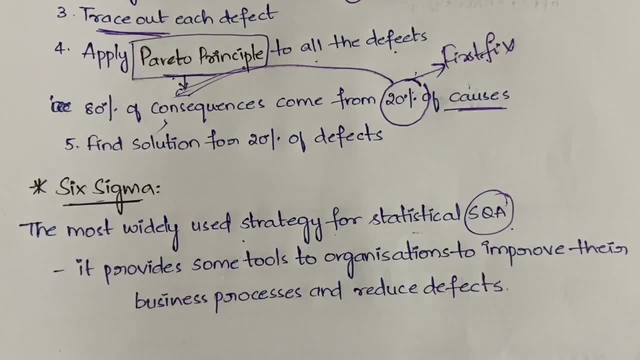 some tools to organizations to improve their business process status in order to improve the quality of the business And also to reduce the defects Got it So? Six Sigma is a strategy which is used by organizations, So it will provide some tools to the organization through which they can improve the quality. 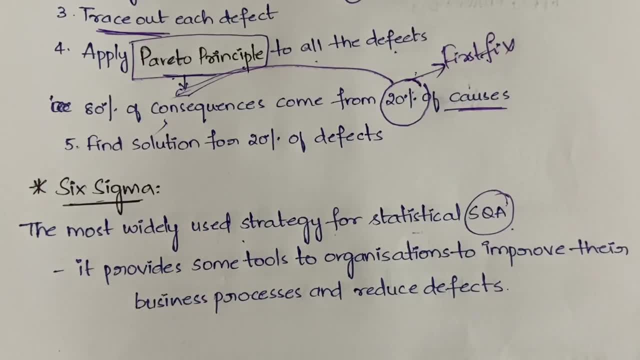 of their organization and, at the same time, reduce the defects. Got it? So that's all for this video. I hope this video is useful for you. If you are still having any doubts, apart from what I have explained in this video, just let me know in the comment section. I